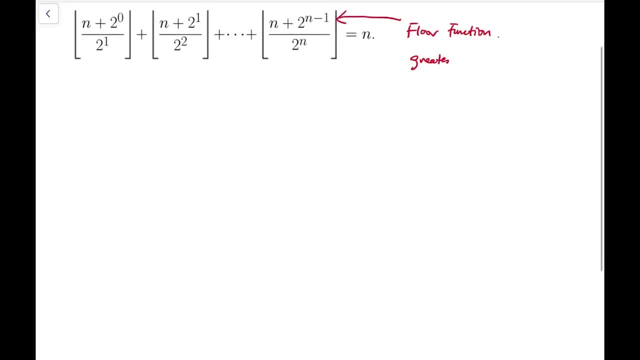 It is just a simple equation. Even though I have so much information, I can still calculate the integral parts, actually referring to the greatest integer that is not larger than the number inside. so of course, if the number inside is positive, then say four point one. of course we are referring to four, and so as, in effect, the integral part. 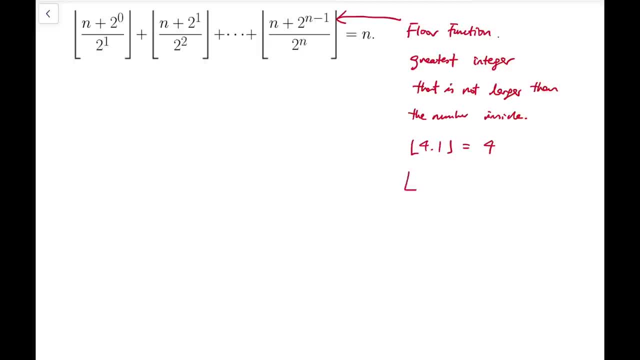 but if we're referring to negative numbers, if we apply this function on negative numbers, say minus three point two, then it's not minus three. well, the integral part of this number is minus three, but the floor floor function of minus three point two is not equal to minus three, is actually minus four, is 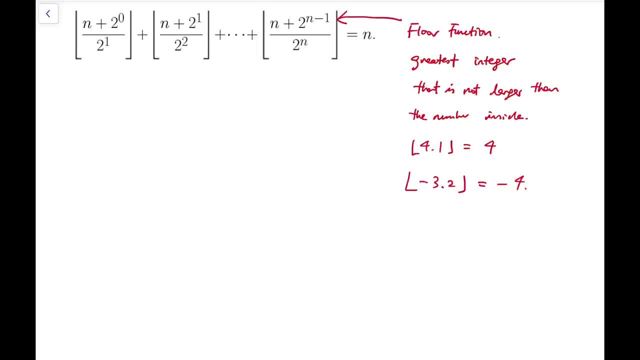 that because only this number fulfills the definition of the floor function. so just to clarify this. now back to the main problem. all the terms in the sum out of the form n plus some power of two divided by the next power of two. so if it's n plus four, that's divided by eight. 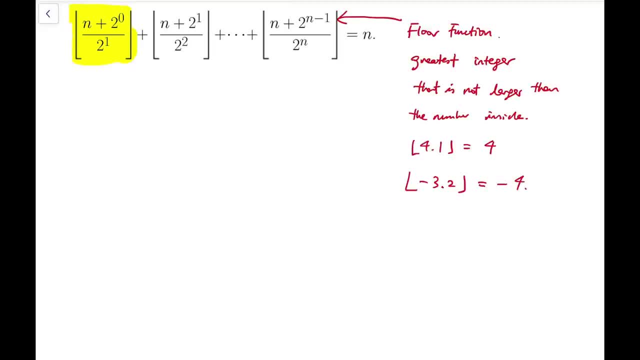 if it's n plus 32 is divided by 64 and so on. so I'm going to say: simplify one of them. I'm getting n plus two plus one half. I'm splitting the fraction. and similarly, for the last term is equal to n divided by 2 to the end, and the fraction either. 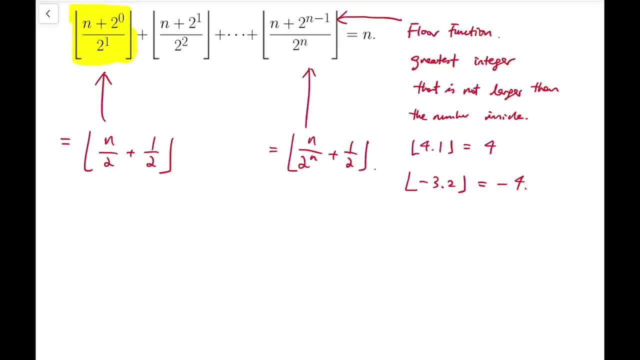 by 1- 3. so the key to solve this problem is to analyze what's going to happen to the after up 1, the floor function. if i add the original number by one half, as in, what would have? how can i simplify this expression? so to do this, i'm going to write: x equals to m plus epsilon, so m is a natural number. 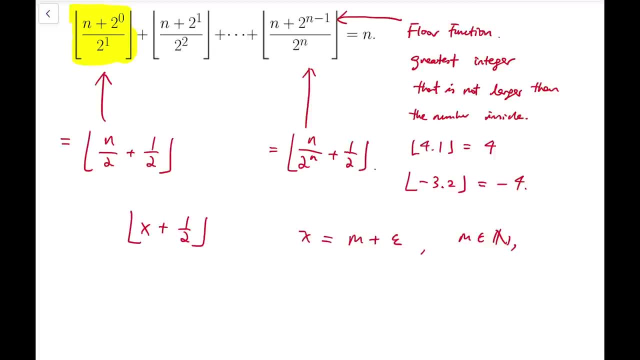 and this epsilon is some number that is between zero and one. we do not take epsilon to be equal to one, so epsilon satisfies this inequality. of course i'm only dealing with positive positive numbers, x, so now i can rewrite this floor function to be m plus a half. 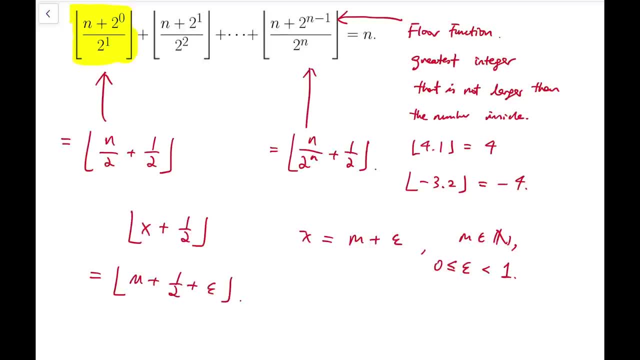 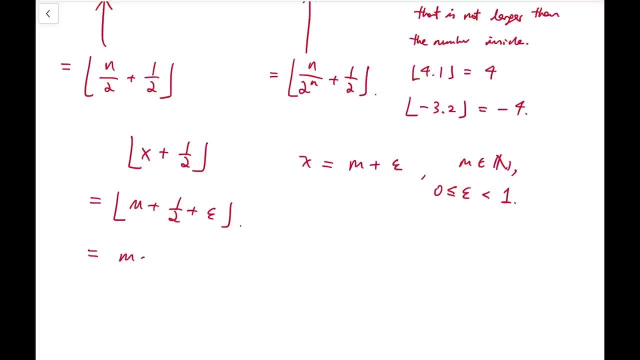 added by epsilon and, of course, by definition of the floor function. i can take out the m because m itself is a natural number. so it suffices to consider what's going to happen to one half plus epsilon. for this i'm going to divide into cases. again, i'm going to divide case into: 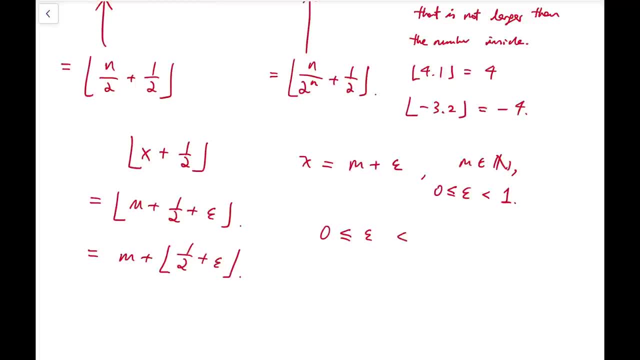 epsilon to be between 0 and a half, where epsilon is not taking the value of a half. where, for the second case, epsilon is between 1 half, taking the value of 1, half this time, but still less than 1. so this is the first case. 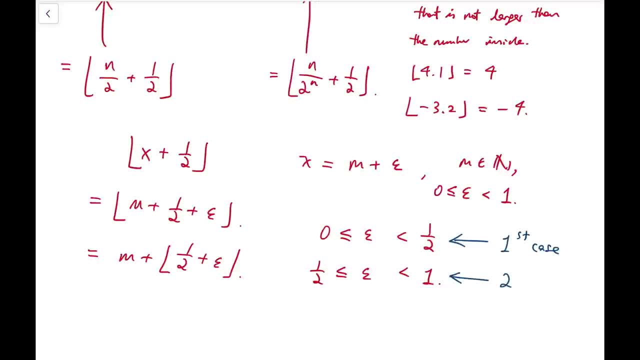 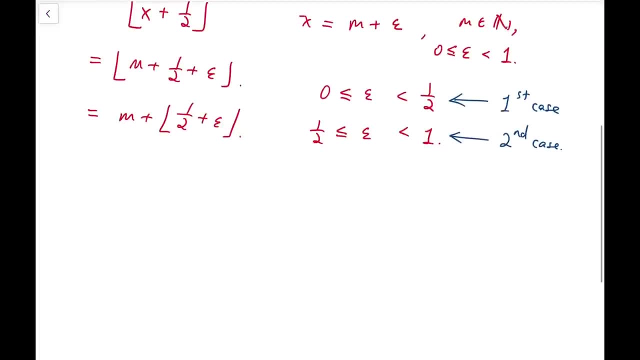 and this is the second case. now for the first case, case 1, I should say that 1 half plus epsilon is between 1 half and 1. most important point is that it's less than 1, so that means it's it's it's less than 1. 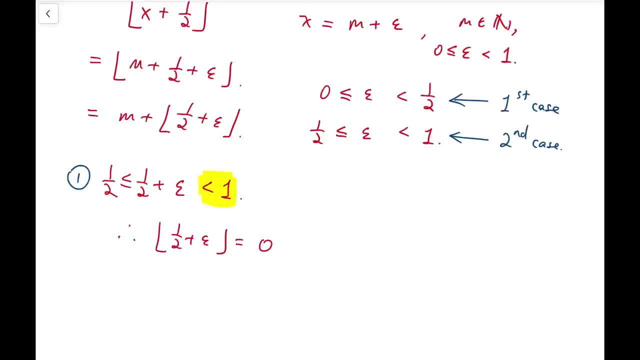 if I apply floor function on this number, it's equal to 0, so then it's equal to m, while for the second case the different thing is that this lower bound becomes not 1 half this time, but 1, and the upper bound is 3 halves. 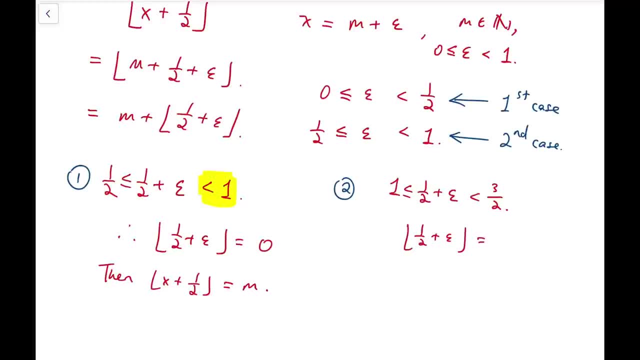 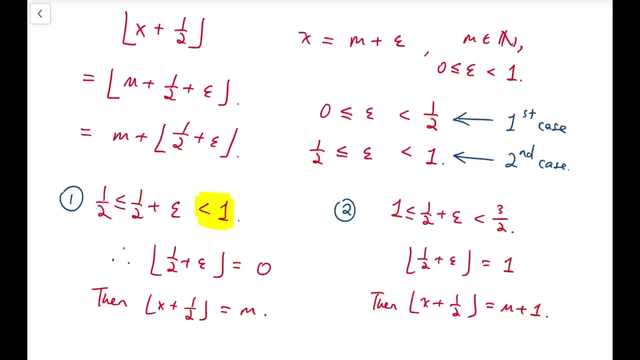 and so floor function of a half plus epsilon is equal to 1. now, for this time, the floor function of x plus a half is equal to m plus 1 instead. now here comes the trick. so we know that to simplify the floor function of x plus 1 half, 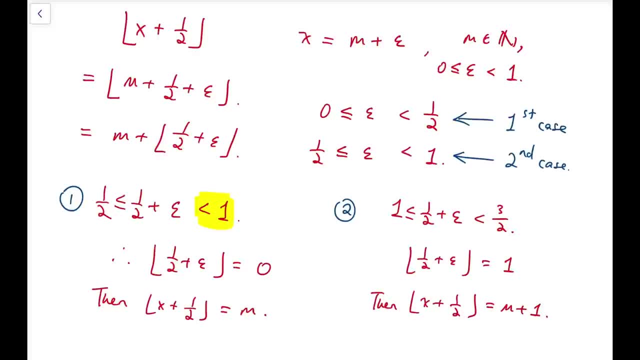 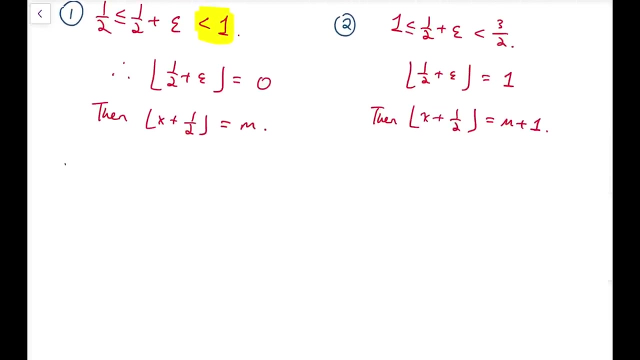 I need to divide the decimal part, which is epsilon, into two cases and for each case the interval of the inequality above 1 half. so to display this effect I'm going to double x, so notice that 2x can be written as 2m plus 2 times epsilon. 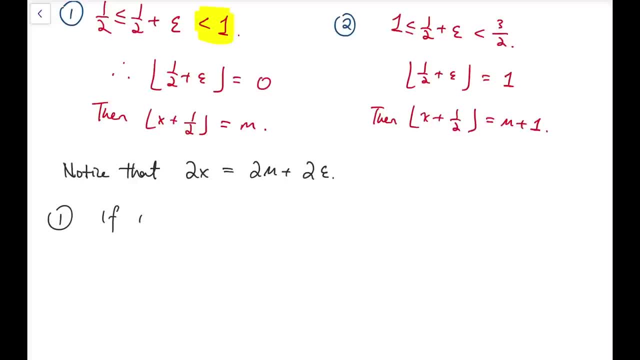 now, for the first case, if epsilon is between 0 and 1 half, then if I double it, it will be between 0 and 1, so covering the entire range that its floor function would take the value 0, and while for the second case, if epsilon is between 1 half and 1, 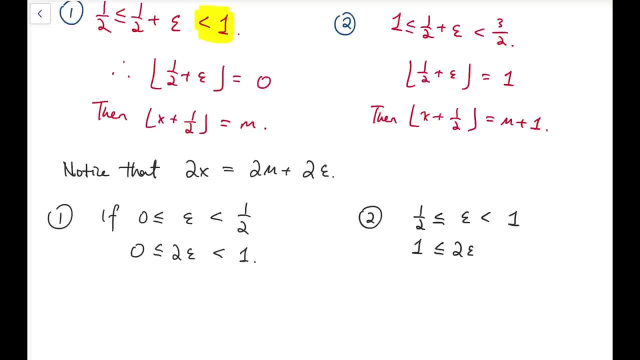 if I double it, it is equal to: the lower bound is equal to 1 and upper bound is 2, so again covering the entire range of numbers having floor function. taking the value of 1 now, the difference will then be displayed. so now, under these two cases, 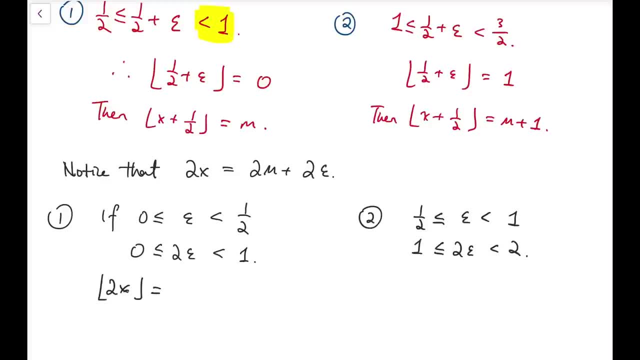 2x. we then take 2m plus the floor function of 2 times epsilon, and that's 2m. and while for the second case 2x is the same, is equal to the same expression, but this time taking the value 2m. 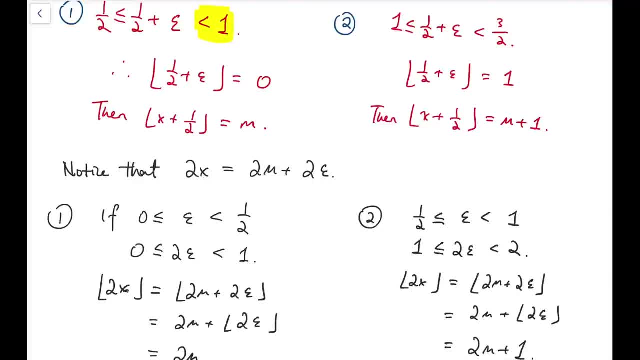 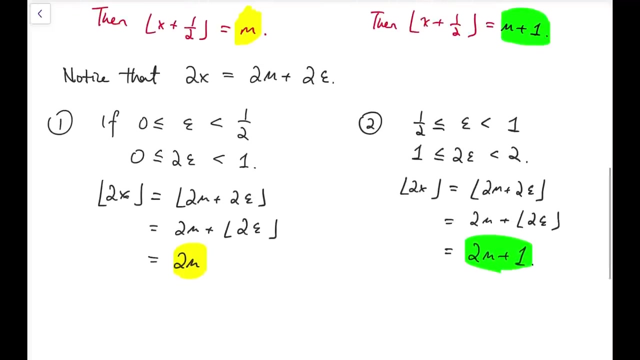 plus 1 instead, so comparing 2m versus m, while for the second case we are comparing 2m plus 1 versus m plus 1. so they differ. both differ by m. so I'm going to say that, regardless of both cases, 2m plus 1. 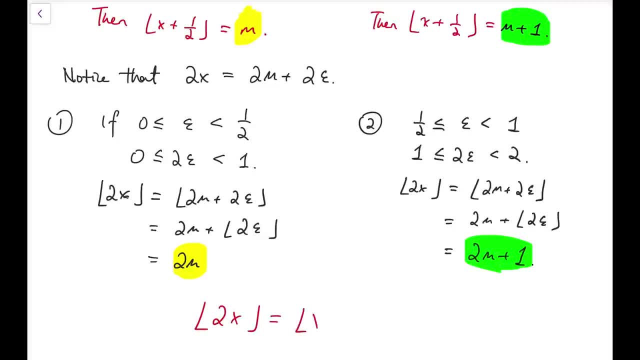 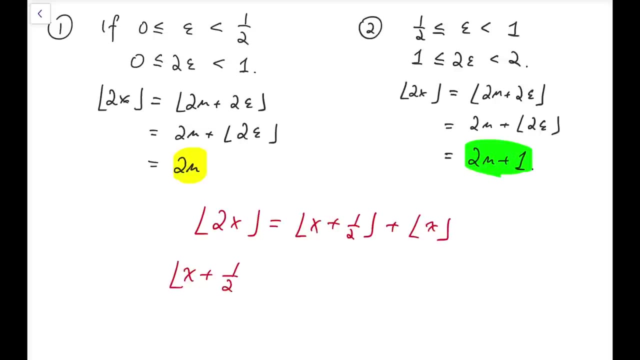 is equal to 2x. the floor function of 2x is equal to the floor function of x plus 1 half added by m, and m is actually the floor function of x. so I have a very nice identity, which is that the floor function of x plus 1 half. 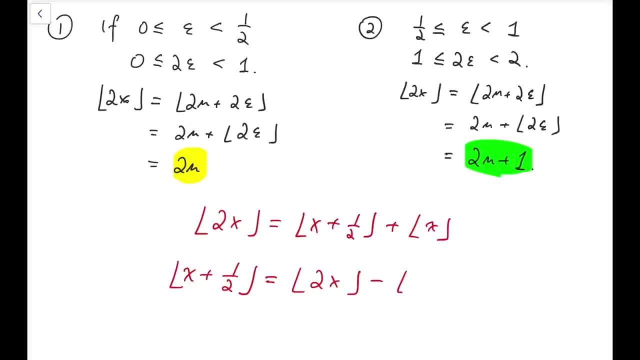 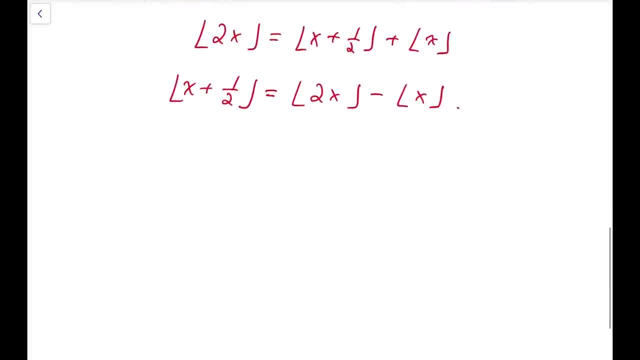 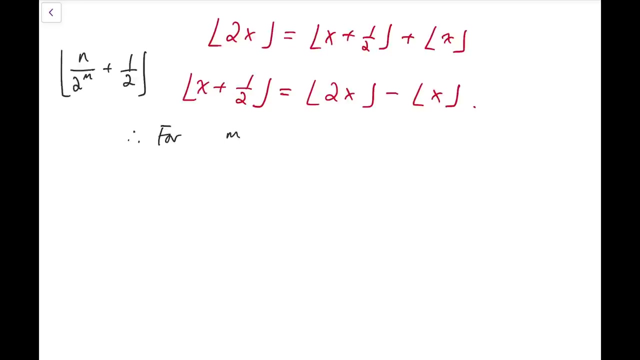 can be written as 2x minus x. now back to the main problem. so we are adding stuff of the form n over some power of 2 added by 1, half. under this identity I can say that for m to be between 1 and n. 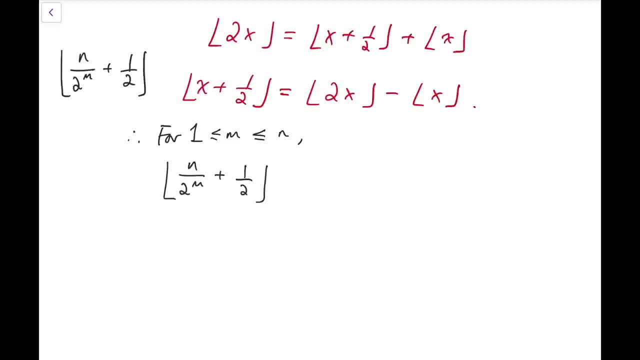 floor function of n over 2 to the m added by 1 half equals to 2 times n over 2 to the m subtracted by the floor function of n over 2 to the m. simplifying we get floor function of 2n over 2 to the m minus 1. 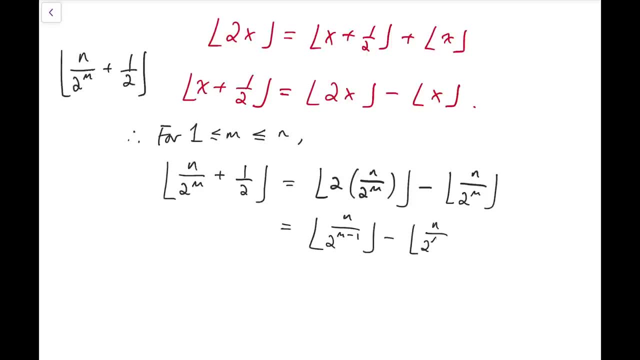 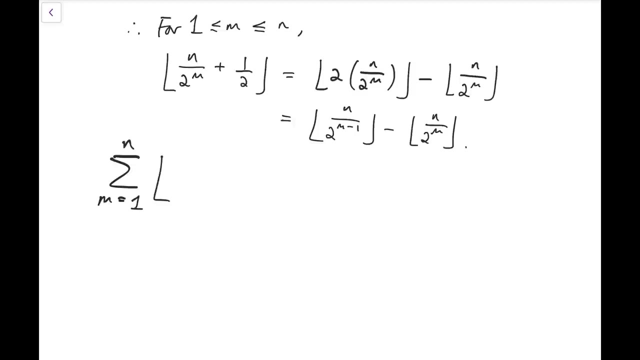 subtracted by the floor function of n over 2 to the m. now our sum in the original problem is adding all terms of the form n over 2 to the m. added by 1, half the floor function of it from m equals 1 to n. 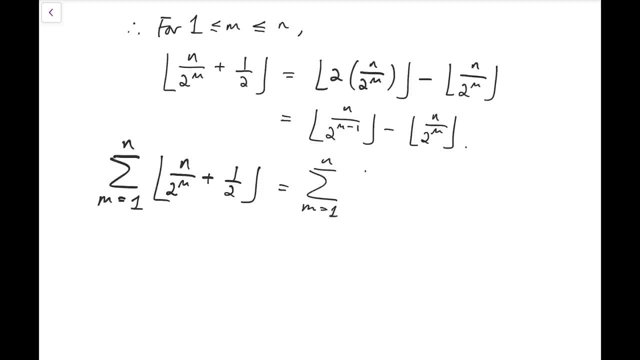 and it's equal to the difference that we have got just now and notice that it's actually a telescoping sum. so say, for the first term, we have n over 2 to the 0 floor function, minus n over 2 to the 1 floor function. 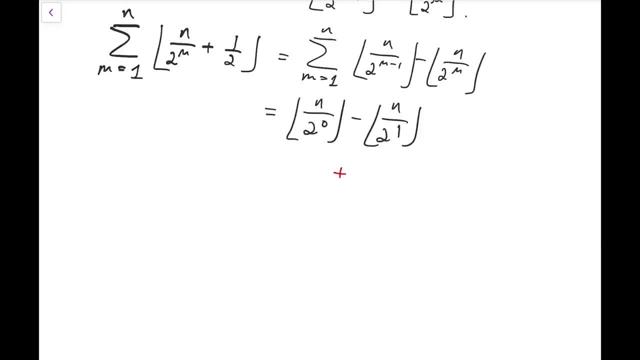 while for the second term we get plus n over 2 to the 1 floor function, minus n over 2 squared floor function, we can see that the n over 2 terms cancel out. we can do similar things for the next term, added by n over 2 squared. 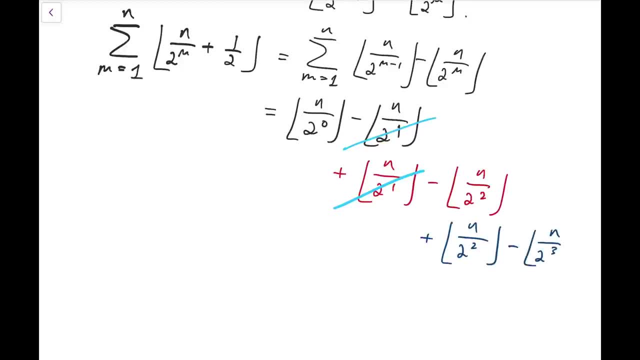 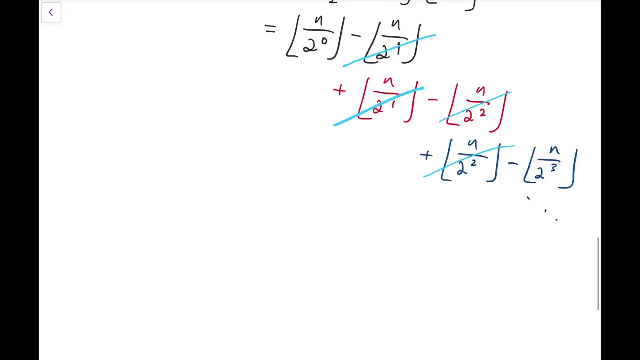 floor function minus n over 2 cubed, n over 2 cubed, n over 2 cubed floor function and the 2 squared term, n over 2 squared terms cancel out as well. so if we keep doing this, at last I'll eventually get. 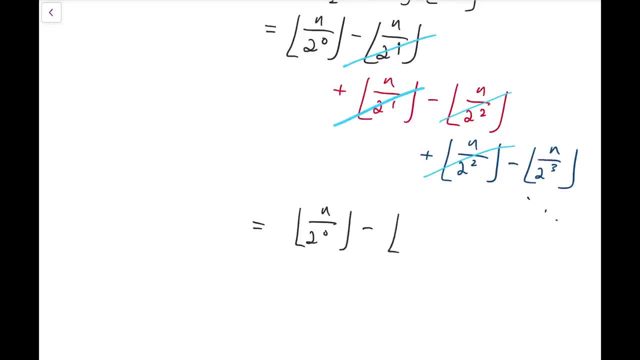 the floor function of n over 2 to the 0, subtracted by the floor function of n over 2 to the n, now 2 to the 0 is just 1. so we have the floor function of n and that's actually just n. 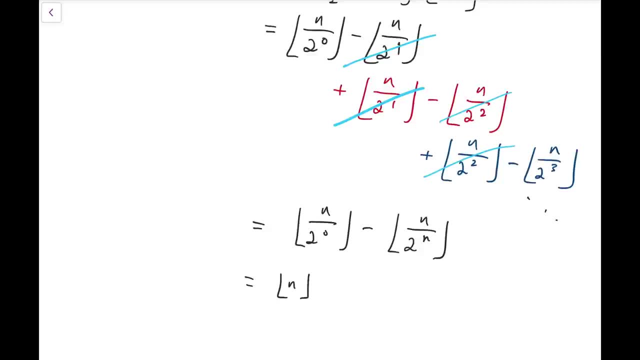 because we've defined at the beginning that n is a natural number and this term subtracted by n over 2 to the n floor function of n, and we know that starting from n equals 1. let me construct a table. so, when n is 1, 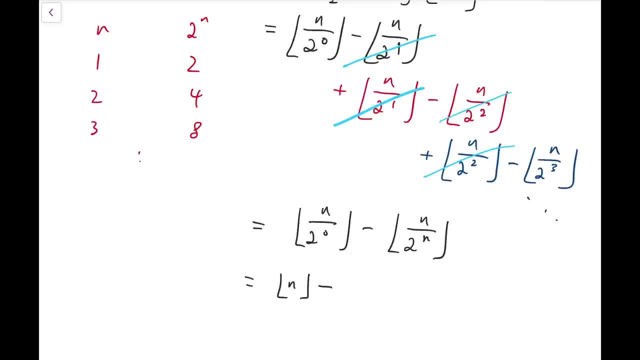 2 to the n is 2, when n is 2, 2 to the n is 4, 2 to the n is 3, 2 to the n is 8, and so on. so we know that when n goes to the next number, 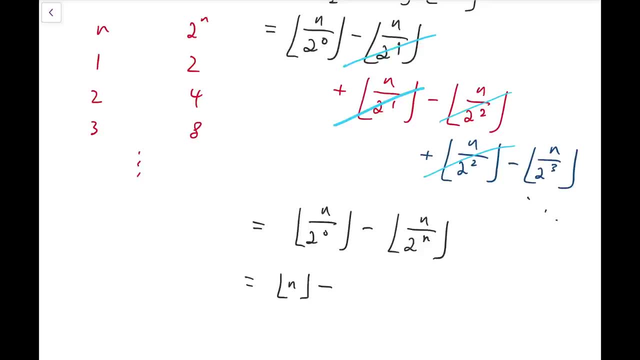 is increased by 1, 2 to the n doubles. so 2 to the n definitely increases faster than n. but I'm not going to like prove it very carefully here, it's just calculus. so we know that n is definitely smaller than 2 to the n. 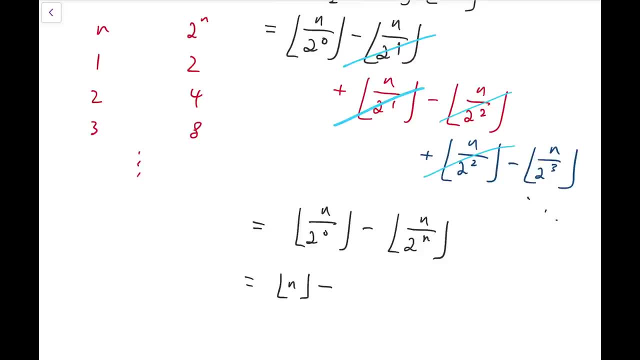 for any natural number, n, so the floor function of that number must be 0. so we've got what we want. the sum is equal to n. so this is the end of the proof.